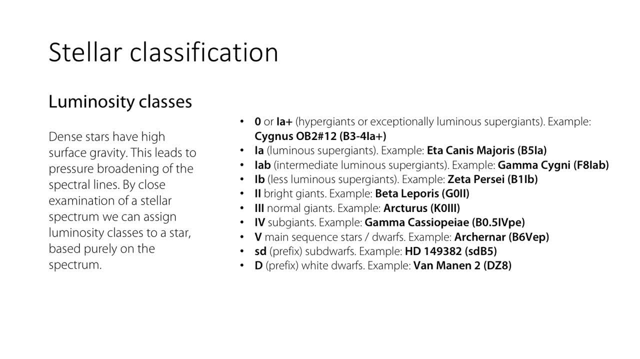 bunch of information that comes from that and its luminosity class. So stars can be determined in terms of their surface temperature and luminosity. The other piece of information that we looked at in the last class- obviously in the last class- is the mass luminosity. 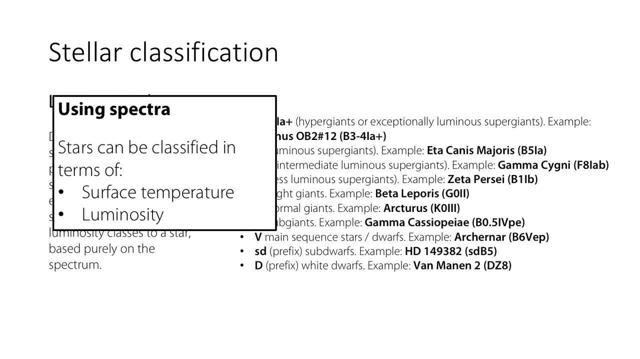 relation- I tried to be pretty clear with this in one of the last videos- was the composition, what the stars are made out of, and now it helps, but that's not SO significant for the purposes of this particular diagram. We really care about the stars' surface temperature. 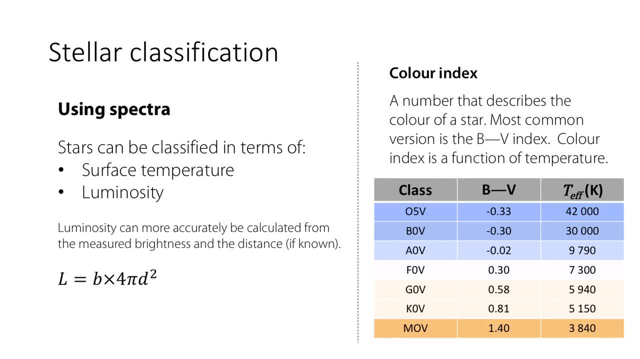 and it's luminosity In terms of the surface temperature and the class of the star. the other piece of information was that the colour of the star changed, and that's important because that's very directly observable If we want to understand mass luminosity. deaths for stars, the one that needs more. 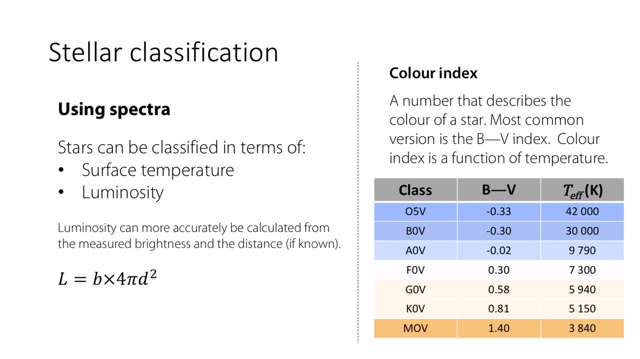 observation is this image here at the top, here at the top of this diagram. The last ruling figure is this one here at the top, with 11US preventing these stars running along the球' accommodated. find the spectrum of the star, then we need to actually take its spectrum, which is a bit. 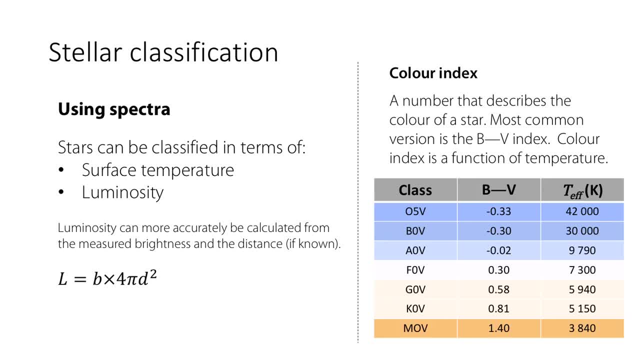 of an involved process. if we can just measure the color of the star, that's a lot quicker and, although there are some some possible pitfalls, it does mean we can very quickly identify the class of the star. so how do we measure its color? we use something called the 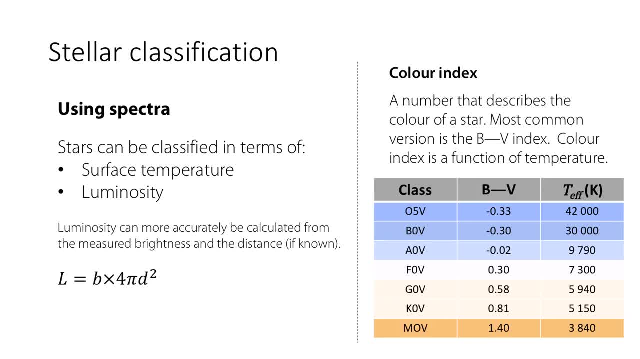 bv index, while there are other versions, but that's probably the most common and traditionally you would take an image of the star in sort of the visual spectrum and then you would take an image of the star just looking at the blue spectrum and by combining the two results and the brightness. 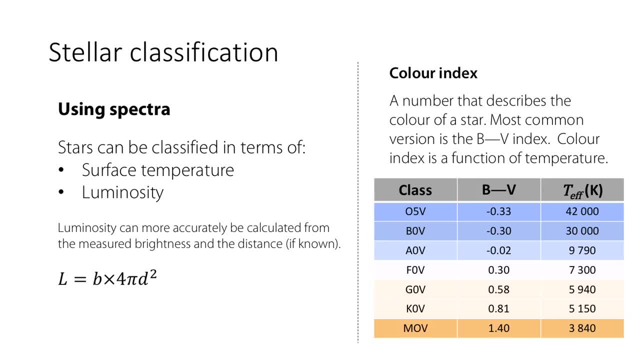 of the star. using those two results you'd see a difference, and that difference is directly related to the color of the star, as you can see in this chart. but just by measuring that, we can know the class of the star and that will also give us the surface temperature of the star. 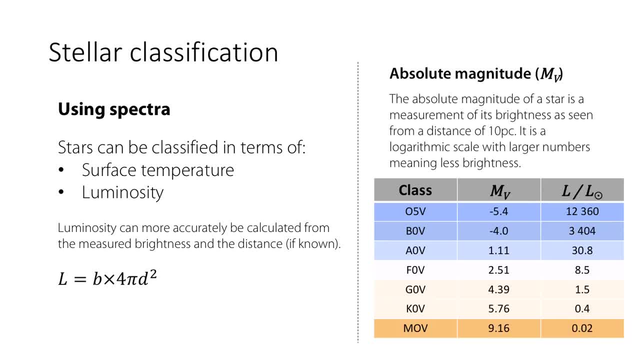 so that's a good way to measure the color of the star. another thing that we did briefly mention is absolute magnitude. this is a you don't, in the current version of this syllabus, need to know much about absolute magnitude. basically, all you need to know is that it is a measurement of the brightness of the star on a scale derived. 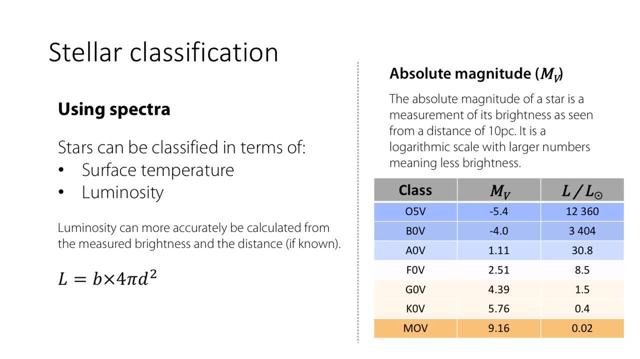 from something that the ancient greeks came up with, but from a uniform distance of 10 parsecs. so it's basically related to the luminosity of the star. so that's a good way to know luminosity. the greater the luminosity, the greater the magnitude, except that magnitude kind of weirdly. 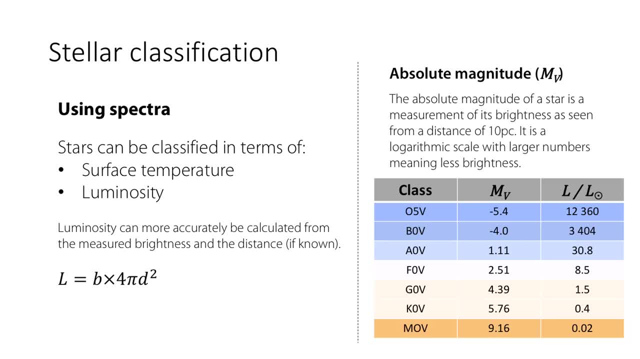 is a negative scale. so the smaller the magnitude, the brighter the star. so minus 5.4 is a very luminous star. the actual brightness as measured on earth of course depends not just on the luminosity and the absolute magnitude depends on the distance of the star from the earth. but as we'll see later, 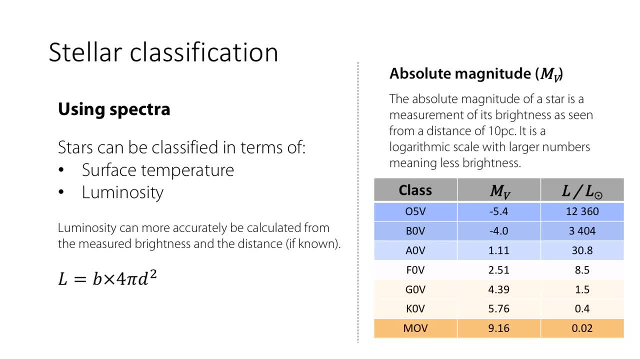 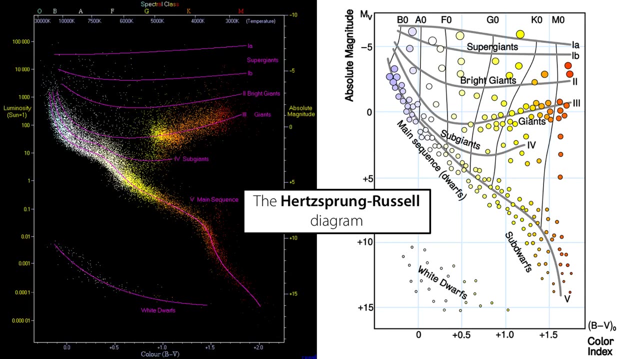 that's an important relationship, because if we know the luminosity, the actual power output, and we know the brightness, what we observe, then we can calculate the distance. that is a very good thing to know. we'll come back to that later. so the hertz from whistle diagram: it's a diagram, it's a chart, it's a scatter plot, is what it is. 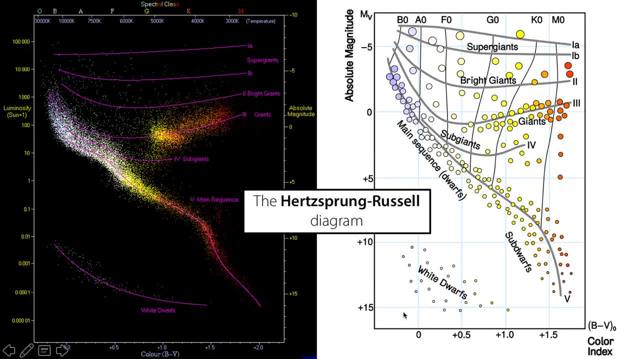 on the x-axis you have. well, both these examples have color index which, as i said, is a useful thing for us to know, because we know the luminosity of the star and we know the brightness of the star astronomers, because it's something you can directly measure, you don't have to calculate it. 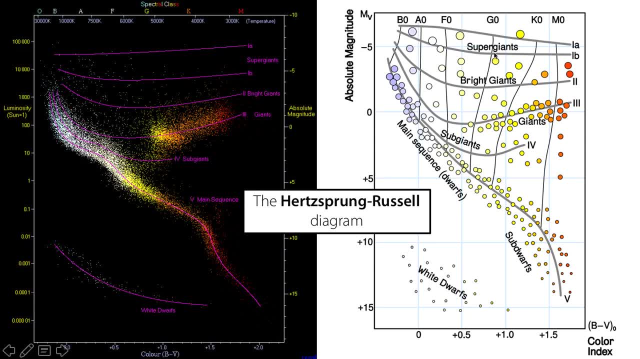 but it's also perfectly valid to have the stellar class, because that's related to the color and, of course, the temperature. the ib, by the way, wants you to know the temperature. it will. if you see a hr diagram or you're asked to sketch a hr diagram, which you may be- then you will have to put the. 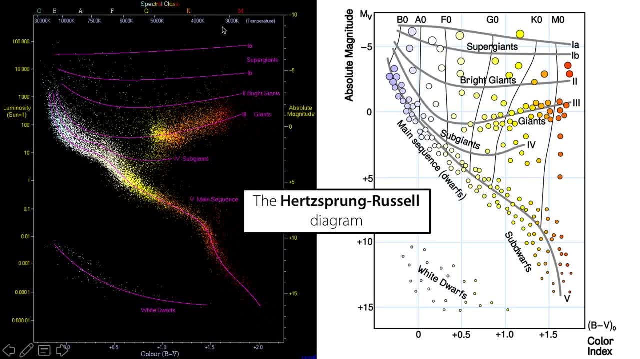 label in temperature, but the key thing here is that the coolest temperature is the temperature of the star which is on the right hand side. for historical reasons relating to relating to the way that the diagram was first drawn, temperature is on the right hand side, smaller, so 3000 kelvin here up to. 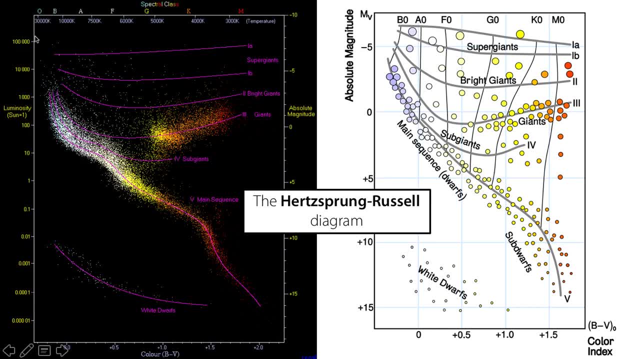 10 and 30 000 kelvin. on the left hand side. the y-axis is made up from one of two different choices, really. one is the absolute magnitude that we just looked at, which is sort of the perceived brightness scale. that's a logarithm of the absolute magnitude, which is the perceived brightness scale. that's a. 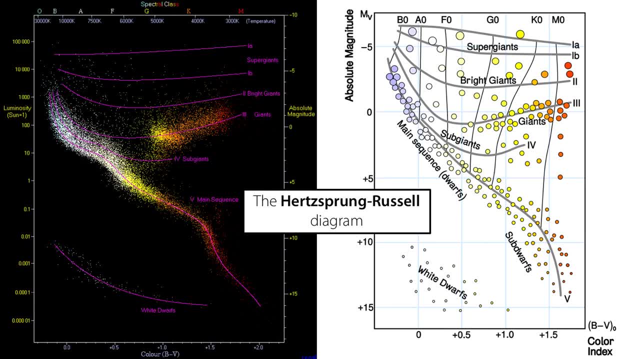 logarithmic scale because it's based on eye response, which itself is logarithmic. or you can put luminosity. luminosity is better. in some ways it's more of an intrinsic property of the star. however, it does mean that you again have to use a logarithmic scale here. you don't with absolute. 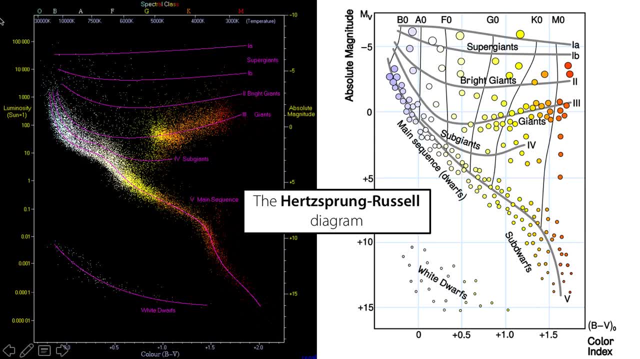 magnitude, because it is already logarithmic, but with luminosity. you must use a logarithmic scale, so one to ten, ten to one hundred one hundred twelve thousand, etc. you do all that, you plot all that and, as you can see in these diagrams there isn't just a random scattering of 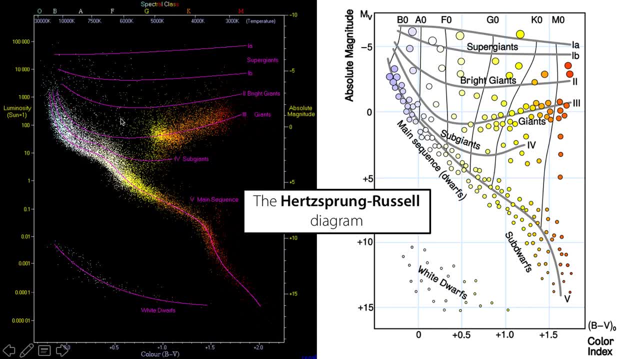 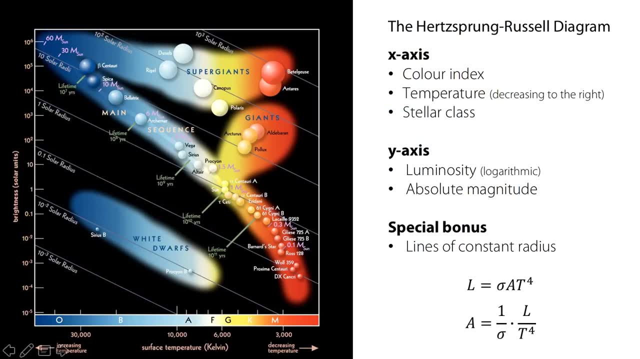 stars. instead they form several clumpy areas. there's another version of that hertsprung russell diagram with actually some named example stars that you could go out and look at in the night sky, although if you wanted to see dx cancri, i think you would need a very powerful telescope. 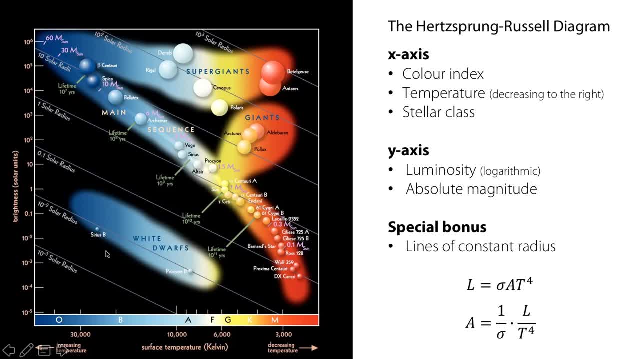 or, for that matter, white dwarfs. but again, on the x-axis, color index, temperature or stellar class. on the y-axis, luminosity, logarithmic or absolute magnitude. as a special bonus, these diagonal lines here are lines of constant radius, so anything along this one solar radius line, which obviously includes the sun. but 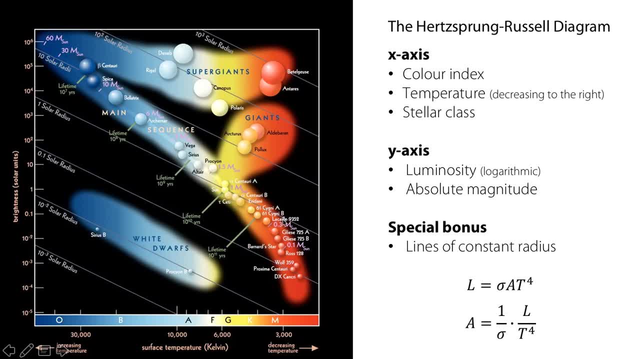 also a few things. a bit smaller than the sun has a radius of the same size as us sun down here and again, this is a logarithmic scale, so this is ten to the minus two or about one percent of the size of our sun is where we find. 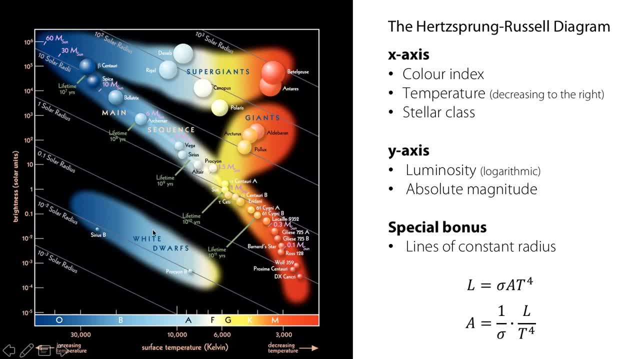 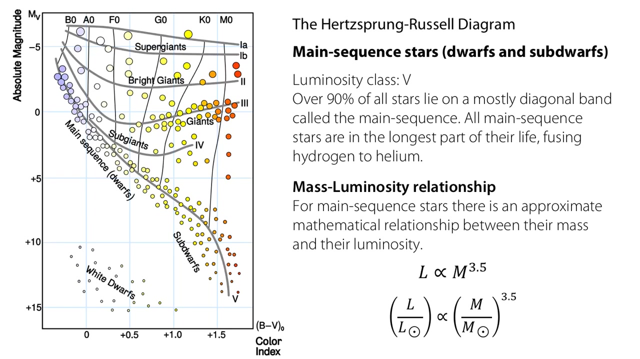 different white dwarfs. the reason we can do that is because the surface area of the star is related by stephan boltzmann law, here to the l over t, to the power of four, and so it's a relationship that we can nicely graph. so what are the different areas of the hertzbrun russell diagram? well, ninety percent of all stars lie on this. 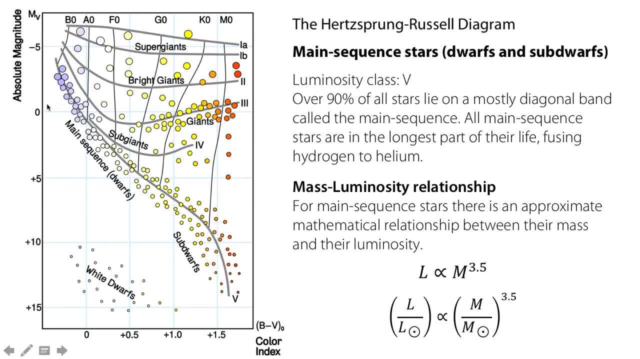 main sequence here. main sequence: stars. luminosity class five stars are all adult stars burning hydrogen into helium. they're actually stars. they're fusing, they're using nuclear fusion. and they're actually stars that are actually fusing nuclear fusion. they're actually stars. they're fusing nuclear fusion. 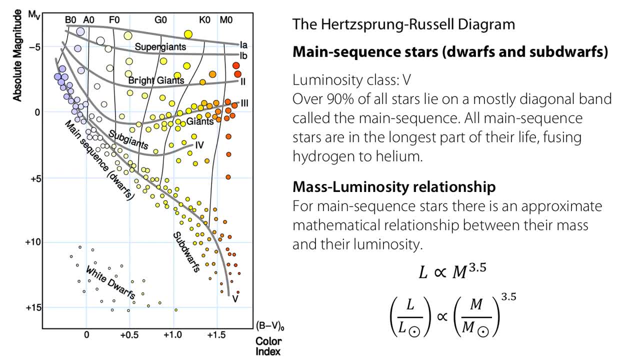 we're using material that's simply not fusing. that's simply not fusing to give power. but that is just the first stage. hydrogen helium: for some it's the only stage. now, obviously, there are my differences between these stars. ever difference between stars is driven by mass. 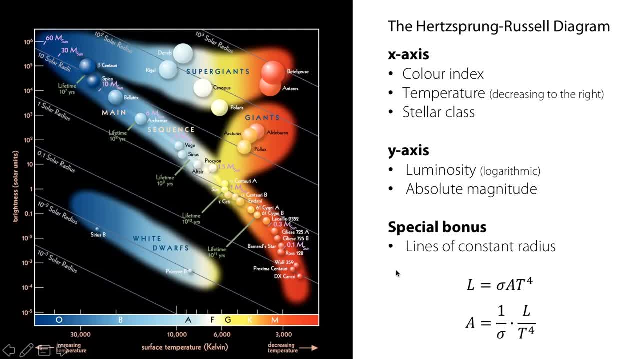 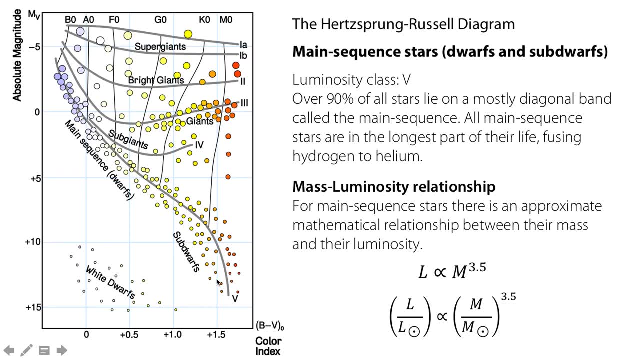 these are low mass, these are high math. one consequence: that 웬. But the low mass stars actually are going to live a lot longer than the high mass stars. They are parsimonious with their use of hydrogen. they only use small amounts of their fuel. 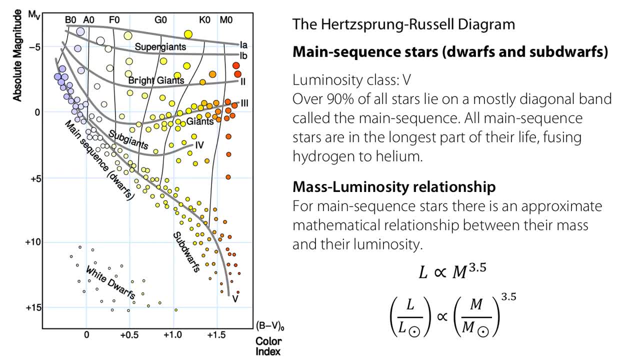 source and also because they're so small, they're very convective. they have big convection currents, which means all of their hydrogen is available for use. A small mass star down here might well spend a trillion years or more converting hydrogen into fuel. Our sun somewhere in the middle here will spend approximately 8,, 9,, maybe 10 billion. 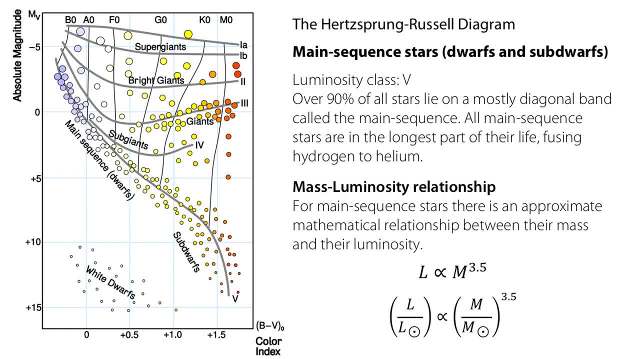 years, 10 billion years. 10 billion sounds a long time, but it's a lot less than a trillion years. The really big stars here, which technically are known as dwarves, even though they have got very high mass, Although actually very small. 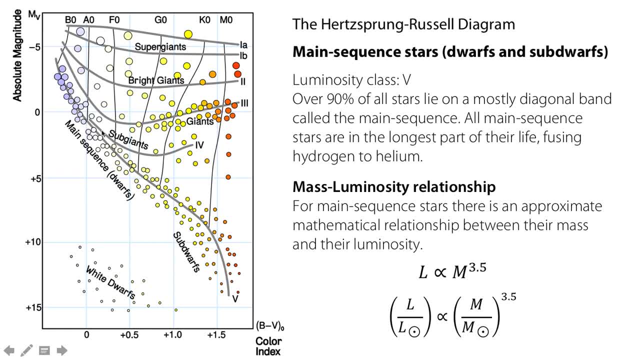 The size. don't forget this diagonal line. the size doesn't grow that much, just a couple of times. These, technically, are known as dwarves. still, they are still main sequence stars, but they will only be on the main sequence for a very short time. 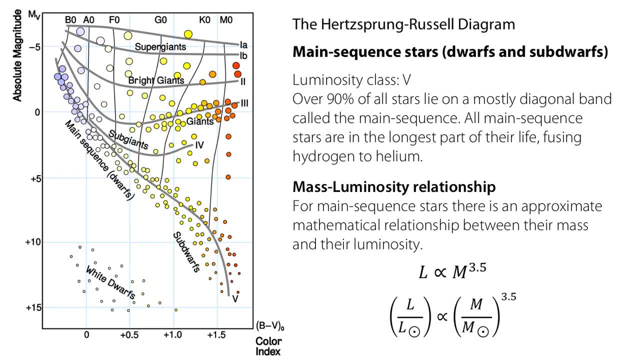 They burn through their fuel at prodigious rates, maybe a million years, maybe even less. But there is a relationship between the luminosity of a star and between its mass and for the main sequence that approximate relationship is: L is proportional to m, to the 3.5.. 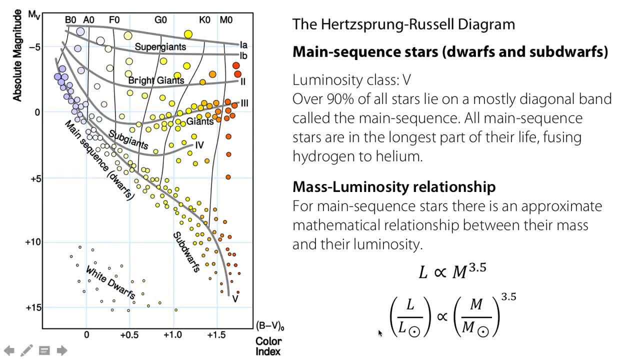 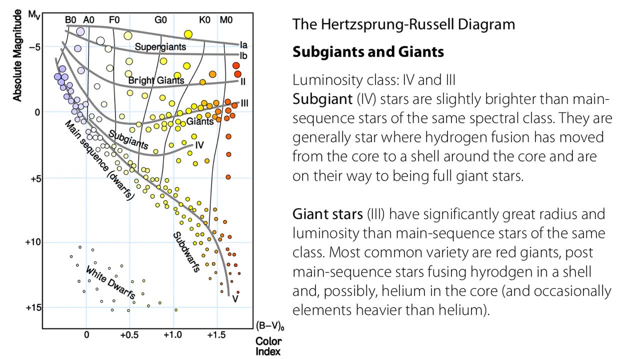 What that means is that a star that is twice as bright of our sun will have a lot more mass than our sun. This is one of the things that the IB needs to know. Conclusion: iny suppliers, we have the sub-giants and the giants. These are no longer main sequence stars. 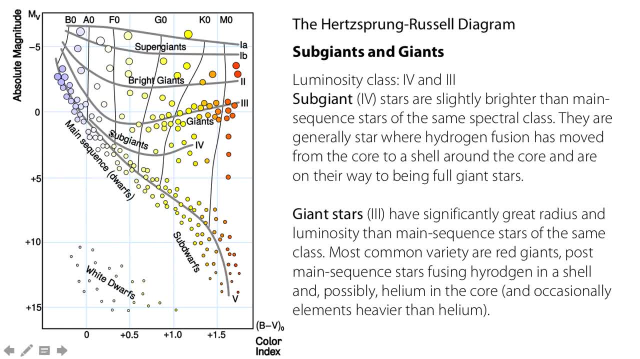 these are post main sequence stars. All of these stars that are not on the main sequence are post main sequence stars. The full details will wait until a future unit, but suffice it to say that hydrogen into helium is no longer happening in the core. That doesn't mean it's no longer happening, it just means it's no longer. 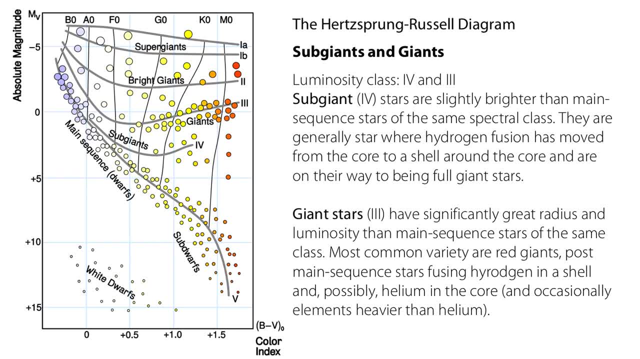 happening in the core. so it happens in a shell around the core, which significantly heats up the outer envelope of the star, which makes it expand, Even though these stars don't gain any mass in the process. in fact, they're losing mass. they become significantly bigger because 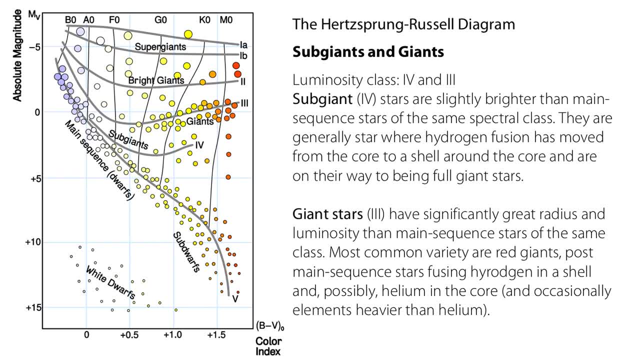 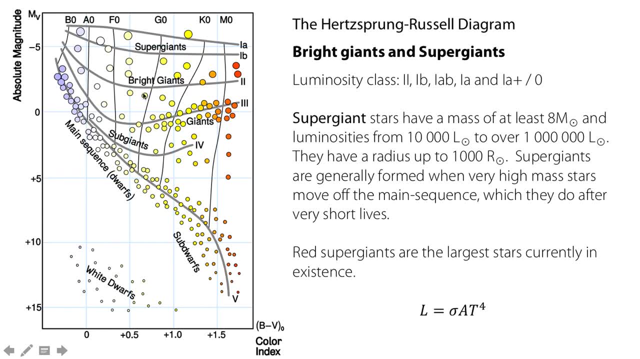 they're significantly bigger. they're also significantly cooler, As I say. well, much more details on this in a later unit. but all these stars up here are giants, Supergiants, which are the largest stars that you can see. some are from a luminosity of a million times the luminosity of our sun and a radius up to a thousand times the radius of our sun. 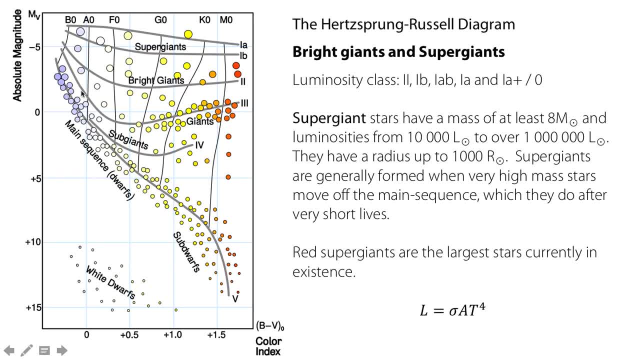 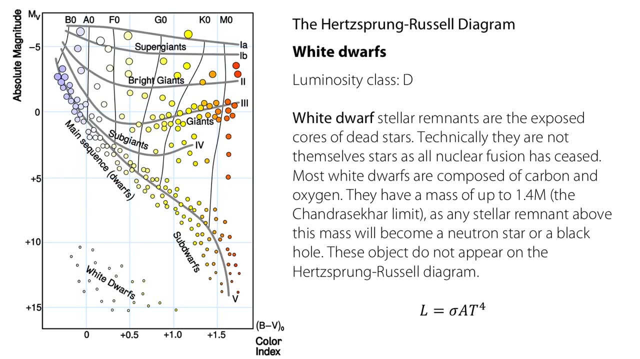 This is the sort of end game for what's already a large mass star when it moves off the main sequence and grows. Red supergiants- remember these diagonal lines representing size. red supergiants are the largest stars currently in existence. On the other part of the scale down here we have the white dwarfs. 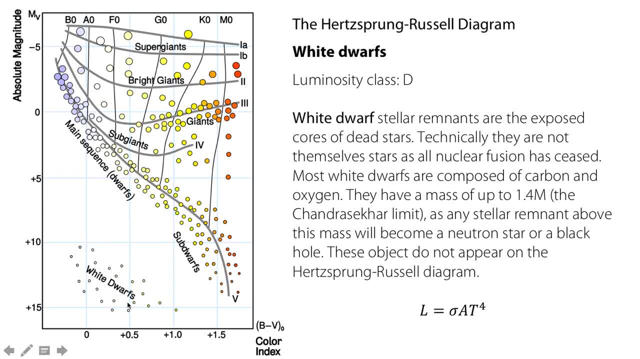 White dwarfs have a very low luminosity, but they do have a very high temperature. So by this equation, if they have a high value of T and yet a very low value of L, they must also have a very low value of A. 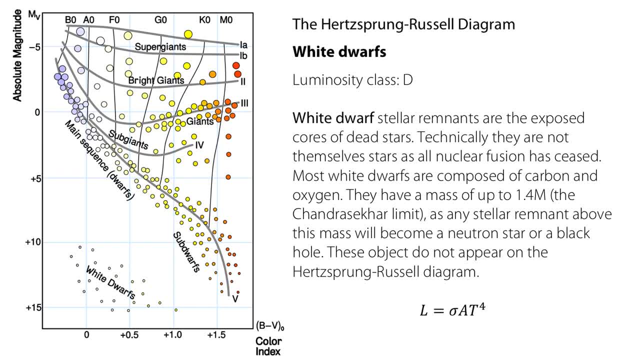 These are very, very, very, very small objects. These are stars, which are, some of them, the mass of our sun, or more Actually, technically they're not stars. They're not stars because they're no longer undergoing nuclear fusion. 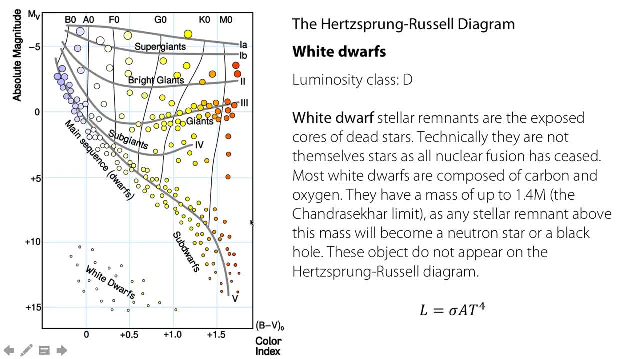 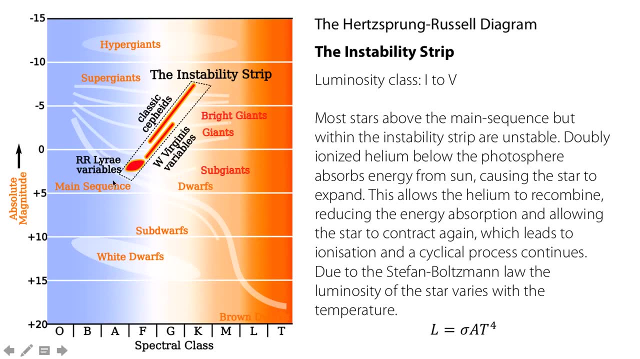 They're stellar remnants, But they're still glowing because they're really hot And even though they have very high temperatures, they have very low luminosities because of their very small size, Probably about the size of the Earth- Another area of the Hertzsprung-Mussel diagram you should be familiar with amongst these other parts that we've mentioned. 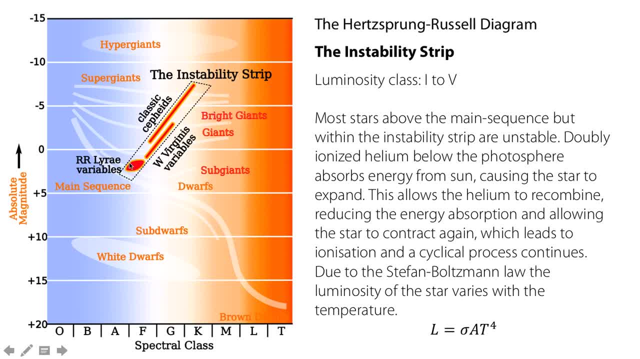 is this area called the instability strip. These stars are again stars nearing the end of their lives which, due to a combination of their composition and their size and their temperature, are variable. They vary in brightness And they vary in brightness, they vary in luminosity by varying in size, actually. 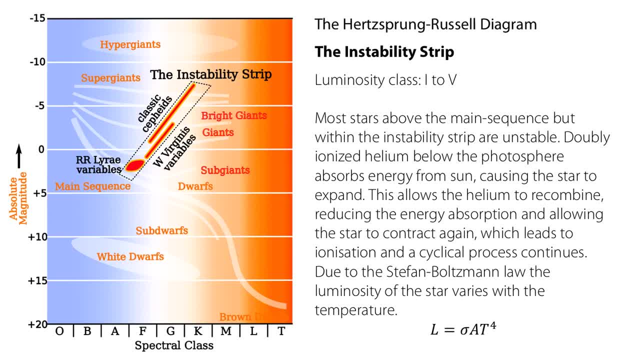 The full details you don't really need to know, But basically there's a feedback process where the star tries to maintain its hydrostatic equilibrium But it fails. Parts of the star absorb energy And as they absorb energy they get hotter. As they get hotter they expand, which causes those parts to change to another form which doesn't absorb energy. 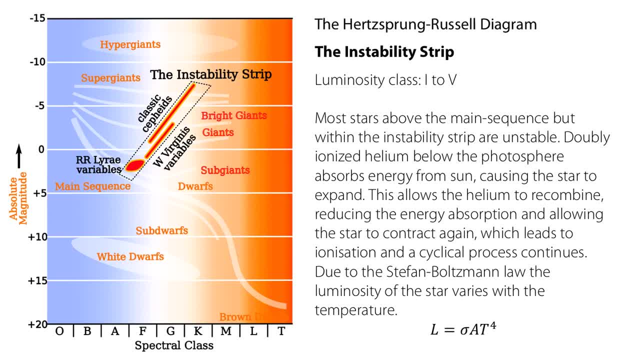 So it contracts, which means that it got hotter, etc. etc. etc. Look at the links in the web pages for more information if you want it. And the application of some of these variable stars is very interesting. So that was a basic introduction to the Hertzsprung-Russell diagram. 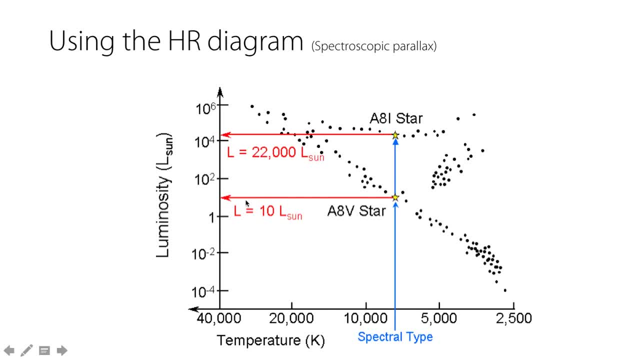 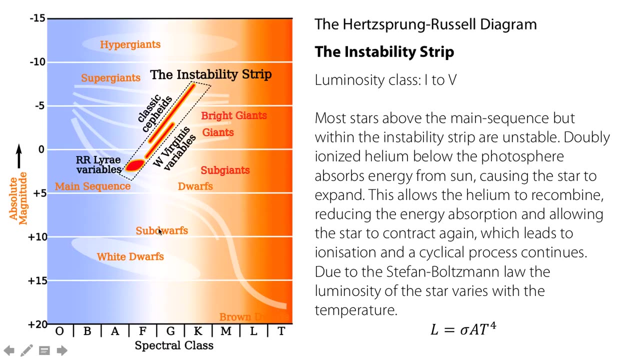 One application of the Hertzsprung-Russell diagram is to actually find the distance to stars, Because if you look at the stellar spectra, you know the temperature and you know the luminosity class. You know: is it a white dwarf, is it a dwarf, is it a sub-giant, etc. 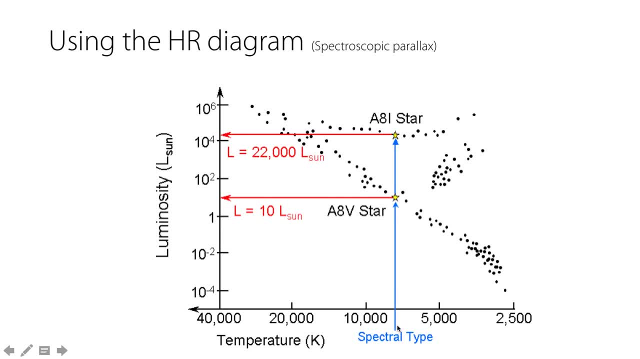 And you can use this information Here. you find the spectral type from the temperature. Okay, it's an A8 star, But is it an A8V star or is it an A81 star, a 5 class 5 star or a class 1 star?